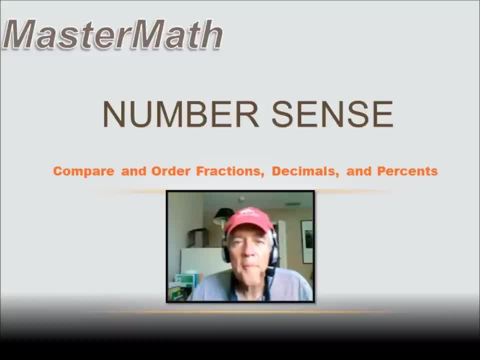 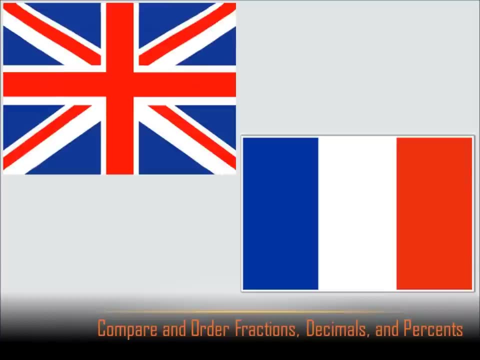 I hope you have a really good time today. Today, we're going to talk about comparing and ordering fractions, decimals and percents, And this is a little bit like translating from one language to another, But instead of translating from English to French, we're going to be translating from English to math. 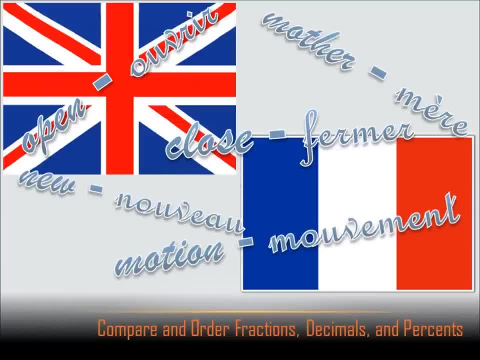 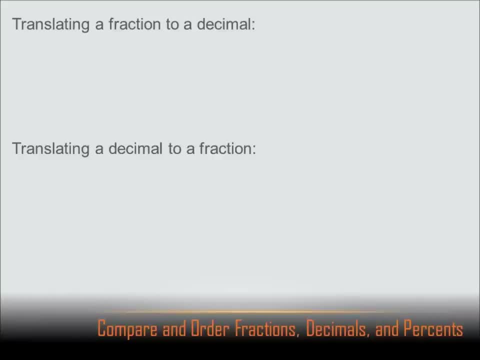 Okay, We're going to talk about fractions, decimals and percentages, And they're all useful concepts, They're all useful tools And they all have different uses. For instance, a fraction. Well, if you had five people in a room and four of them had brown hair, it would be easy. 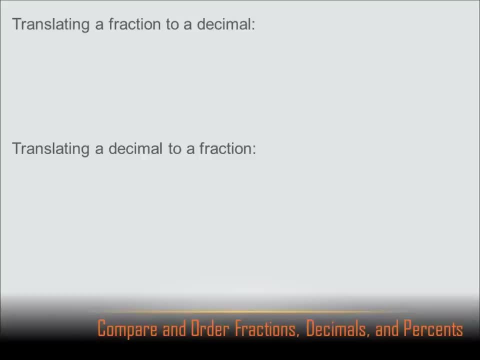 to say that four out of five or four over five was the fraction that represented the people that had brown hair. But if you had five people in a room and four of them had brown hair, it would be easy to say that four out of five or four over five was the fraction that represented the people. 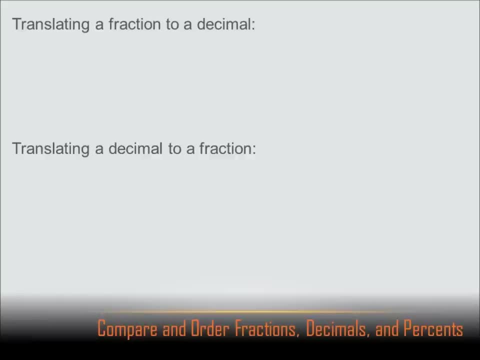 that had brown hair. But if you had a thousand and sixty-two people in the room and you wanted to know how much four-fifths of that was, it would be a lot easier to do that with a decimal, Because .8 times a big number is a lot easier to multiply than a fraction multiplied by that. 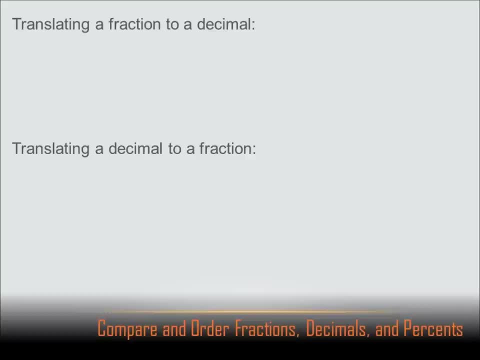 large number, And percentages are really useful too. If I told you that 65% of the people that take math, master math, end up getting an A. it would be a lot easier to do that with a decimal, But if I told you that 65% of the people that take math, master math end up getting an? A. it would be a lot easier to do that with a decimal. But if I told you that 66% of the people that take math, master math end up getting an A, it would be a lot easier to do that with a decimal and you might think I am. 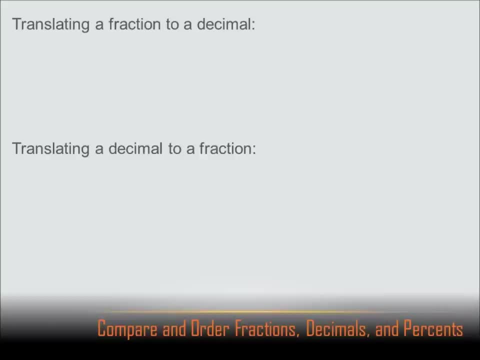 lying, and I might be…but you'd understand what I'm saying. So percentages are really good communication tools within math. Today, we're going to talk about translating between three of the four measurements. First, lets talk about translating a fraction to a decimal. 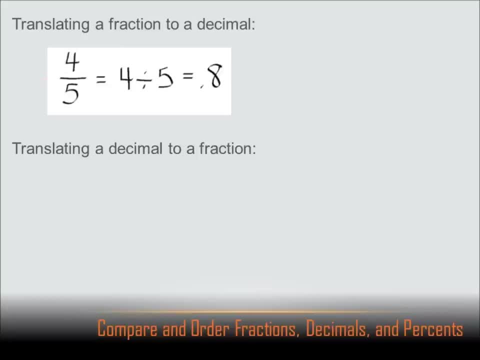 By now. I hope you know that that line you see on the horizon can be interpreted in several different ways ways. We could say that that fraction is 4 fifths. We could also say it's 4 over 5.. We could also say it's 4 divided by 5.. And that's the interpretation I want you to remember. 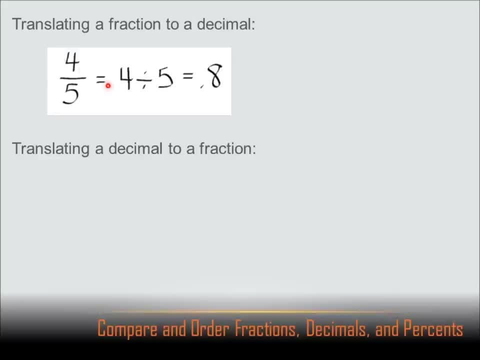 right now, because 4 over 5 equals 4 divided by 5.. And 4 divided by 5 is .8, and .8 is the decimal equivalent of 4 fifths. Well, how about translating from a decimal to a? 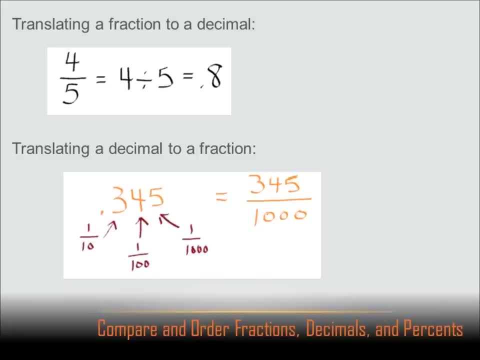 fraction. Well, you know, I hope, by now, that when we have a decimal after the dot, the numbers have place values, That 3 is in the 1 tenth value and that 4 is in the 1 one-hundredths. 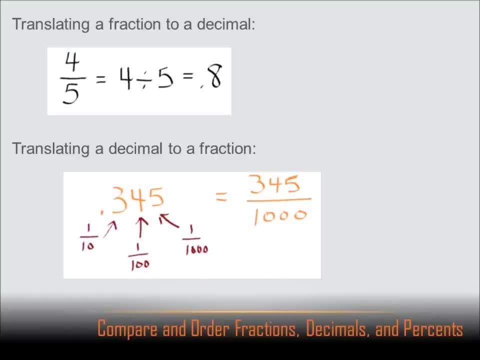 and the 5 is in the 1- one-thousandths And you notice that we just add a 0 to move back 1.. So if I've got .345, the 5 is in the one-thousandths place, so I can change that decimal to a. 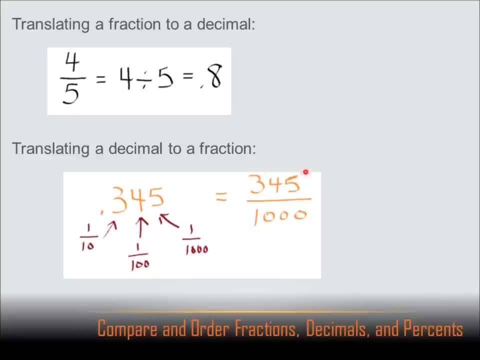 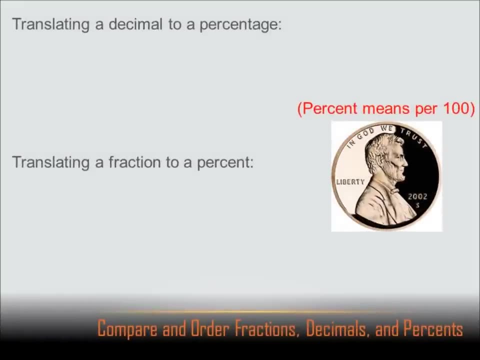 fraction by putting the 345 over a thousand. Okay, well, let's work on changing decimals to percentages or fractions to percentages. It's going to be helpful if you remember that percent is not just an arbitrary word that we pulled out of the air. it means something. Percent means per cent per one-hundred, Because 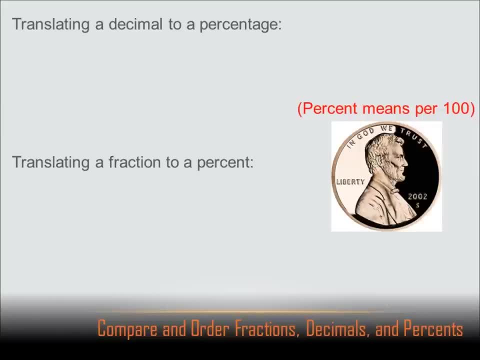 the word cent means one-hundred And the word per means divided by. Remember when we had a fraction 1 over 2, that was 1 per 2.. So that shouldn't be hard to do. It's going to be hard to remember if you remember that a penny is a cent and a cent is one one-hundredth. 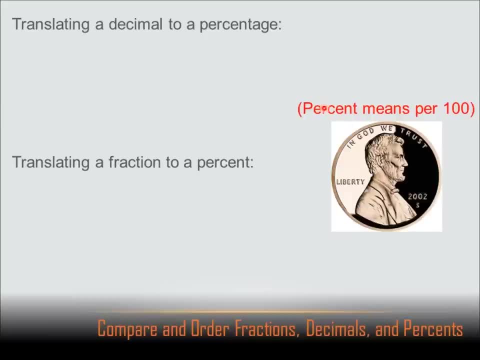 of a dollar. So per cent means per one-hundred. Okay, let's look at converting decimals into percentages, And there's a couple of ways we can do this. I like the second way a lot better, But we could take .62, and we could 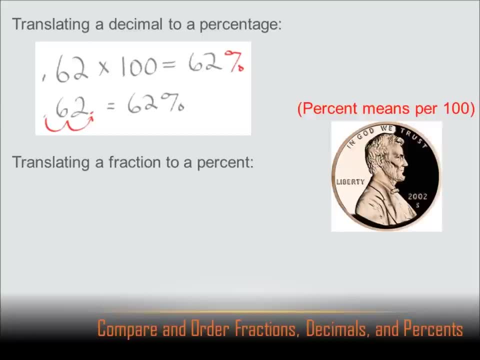 multiply it by a hundred, And if we did that, we'd get 62%. The easier way, I think, is to remember to just move the decimal point two to the right, And then .62 becomes 62%. Well, how about translating a fraction to a percentage? Well, there's a couple of ways. we could do that too. The first way: I'm going to do it in a few minutes. I'm going to do it in a few minutes. The first way I'm going to do it in a few minutes. The first way I'm going to do it in a few minutes. The second way I'm going to do it in a few minutes. The first way I'm going to do it in a few minutes, The first way I'm going to do it in a few minutes, I'm going to show you, You're probably 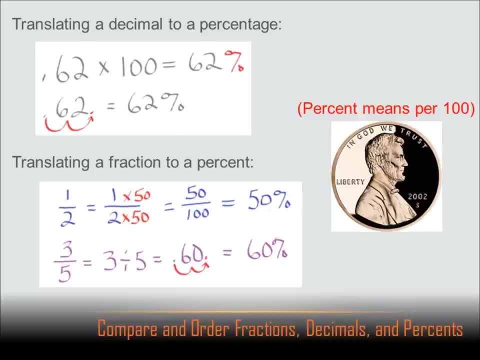 not going to use that often, but it will help you understand a bit about the relationship between fractions and percentages. If I've got a denominator that's a nice, easy multiple of 100, then I can multiply that denominator by whatever will change it to 100.. In this, 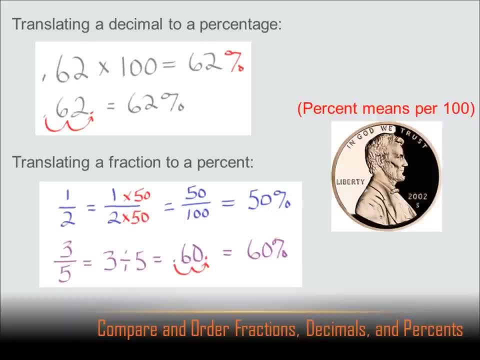 case, 2 times 50 will change it to 100. And then I've got per one hundred or per cent, and the numerator has to be multiplied by 50 as well. so 1 half is equivalent to 50 over 100, or 50 per 100, or 50 percent. Well, I think the second way is going to. 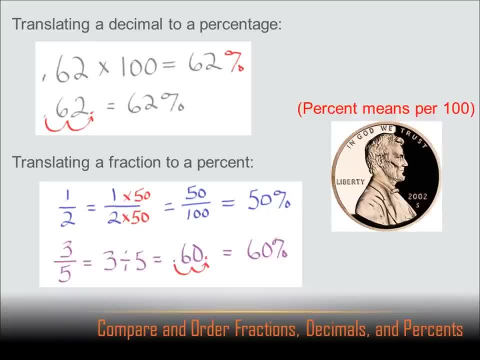 be a little bit easier for you in most cases, and that's to convert the fraction into a decimal- and you remember that 3 over 5 is the same thing as 3 divided by 5, and 3 divided by 5 equals 0.6 or 0.60- and to convert a decimal into a 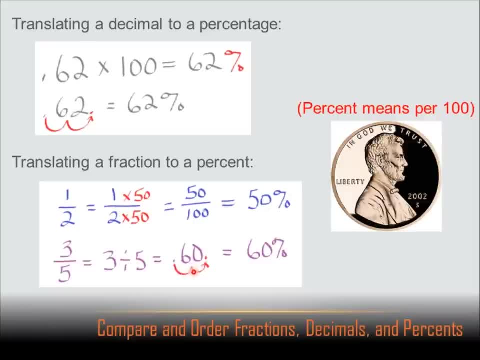 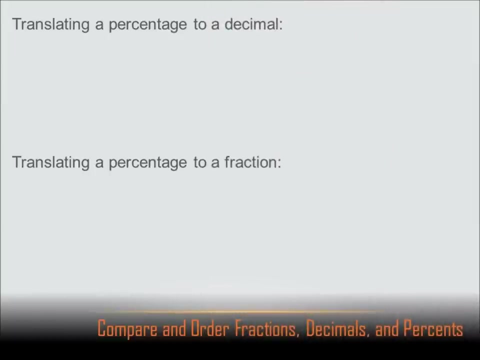 percentage. I just move the decimal point 2 to the right and 0.6 becomes 60, 60 percent, ok, well, how about translating a percent into a decimal or fraction? well, that's not that hard either. let's say I've got 38 percent when I you. 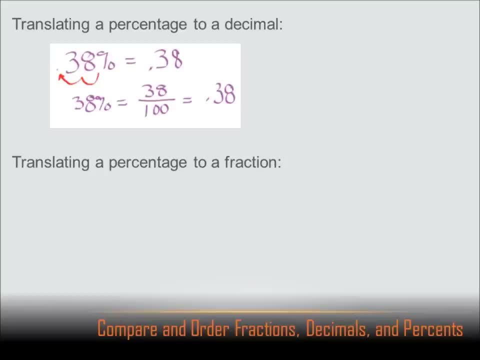 remember, when we converted a decimal to a percentage, we moved the decimal point two places to the right, which was the same thing as multiplying by a hundred. well, if I want to change a percent to a decimal, I just reverse that process. I move the decimal point two to the left and I get. 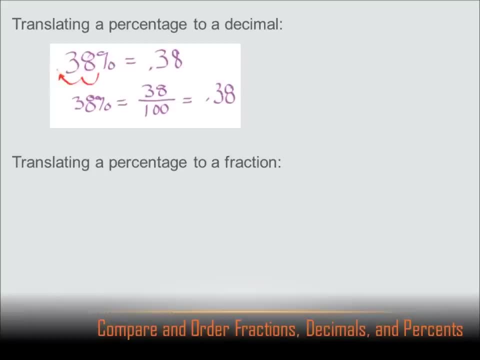 0.38, which is equivalent to 38 percent. here's another way you can do it, although I like the first way easier. I do. I think it's easy to move those decimal points. you just got to remember which direction you move them in. let's say I've got 38 percent again and I want to change that into a percent, or 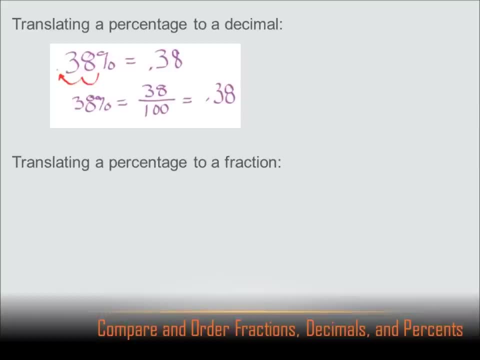 into a decimal: 38 percent is 38 per 100, so it's 38 over 100, and 38 over 100 equals 0.38, while about changing a percent to a fraction: well, that's not that hard either, remember. 42 percent, that's 42 per 100, 42 over 100, and I can simplify: 42 over a. 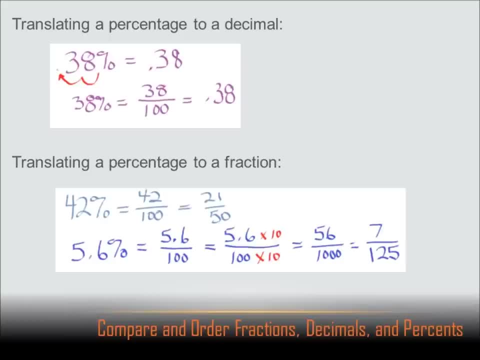 100 to 21 over 50.. I just divided the top and the bottom by 2, and I got 21 over 50.. How about the second one? I've got 5.6% and I want to change that into a fraction. Well. 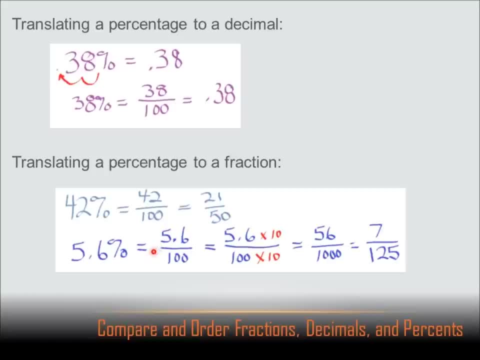 that's 5.6 per 100, so it's 5.6 over 100.. Well, 5.6, that's kind of an awkward number to have in a fraction. So to get rid of that decimal point, I need to multiply the 5.6. 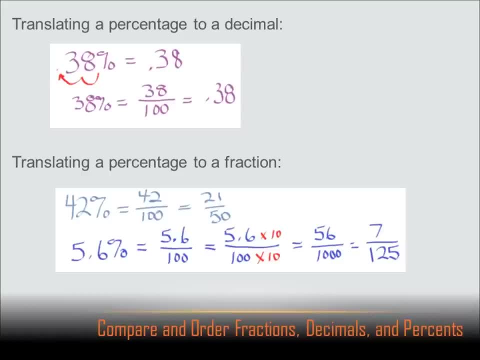 by 10.. And if I'm going to multiply the top of the fraction by 10,, I've got to multiply the bottom of the fraction by 10.. So now it becomes 56 over 1,000.. And I can simplify. 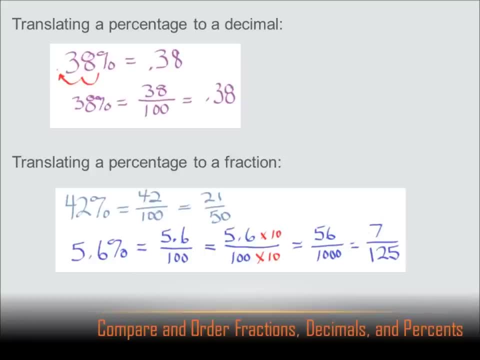 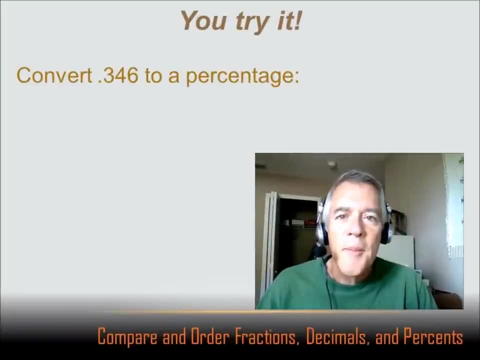 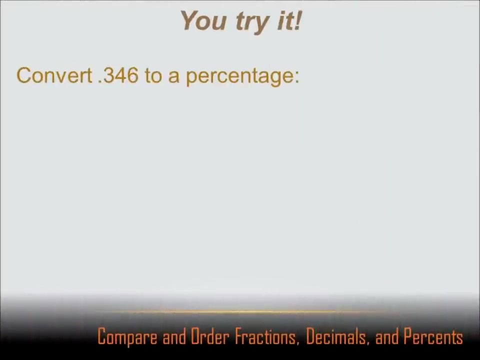 that to 7 over 125.. Now you try this one. Hit the pause button, Do the problem and then hit the forward key to move on to the answer. Convert .346 to a percentage. Hmm, what do we do? Oh, I remember If we're going to convert. 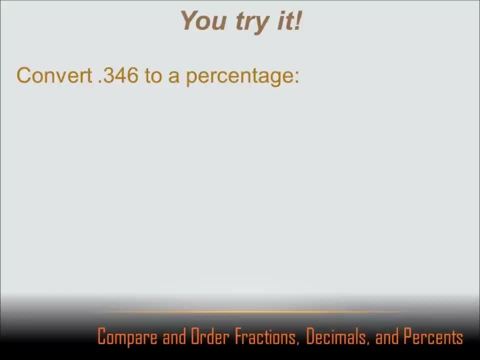 a decimal to a percentage. we multiply it by 100, or we move the decimal point 2 to the right, So I've got .346.. I move the decimal point 2 to the right and I get 34.6%. 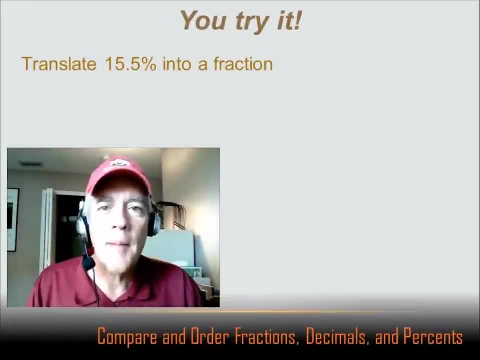 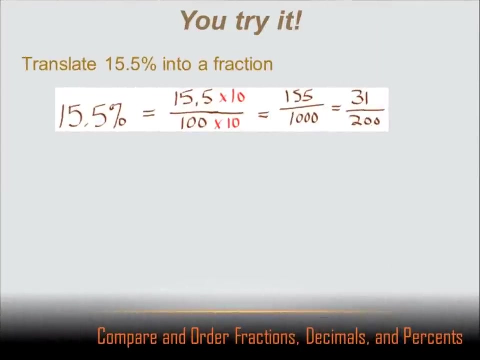 Try this one: Hit the pause button, Do the problem and then hit your forward key. Okay, I need to translate 15.5X percent into a fraction. Well, 15.5 per cent is 15.5 over 100.. But again, 15.5, it's weird. 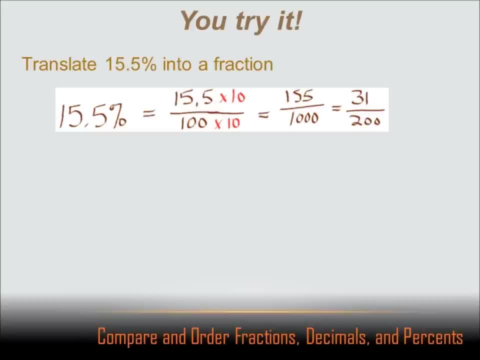 to have a decimal in a fraction. so let's get rid of that by multiplying by 10.. And I need to multiply the top and the bottom by 10, and I end up with 155 over 1000, which I can simplify to 31 over 200.. There's another way I could do this: 15.5 per cent, Well. 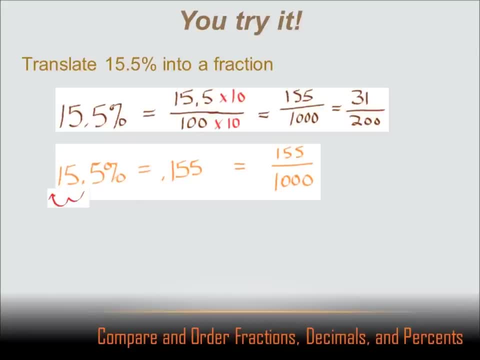 I can move that decimal two to the left and 15.5 becomes .155.. Now that 1 is in the 10th spot, the 5,, the first one is in the 100th spot and the second. 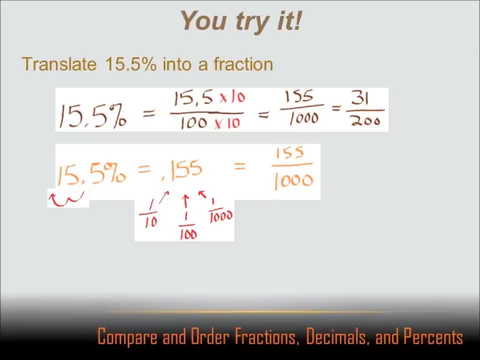 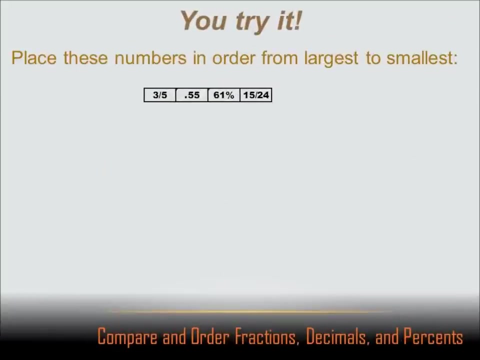 one is in the 1000th spot. So I can change the decimal .155 into a fraction that is 155 over 1000.. Okay, So I've got 155 over 1000.. So what we do? we use the formula of Tier 1 and Tier 2.. We take the number of. 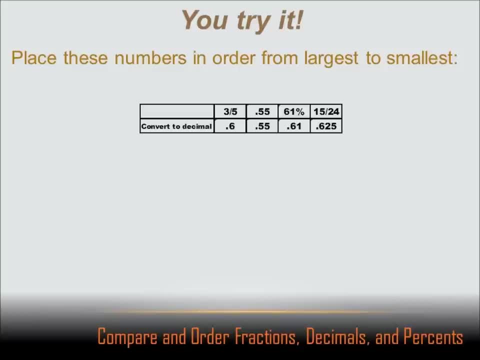 fractions and put them into fractions. We put them all in some wavy format so we can compare them. We can put them all into fractions, we can put them all into decimals and we could put them all in percentages. and in any of those three cases then we could compare. 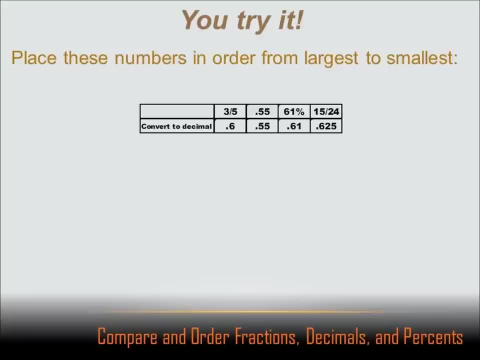 them pretty easily, But they're harder to compare if they're in the mixed types. So all and, let's convert them to decimals, and you'll find that decimals are usually the easiest form to work with. so first, 3 fifths, what's that equal? well, we. 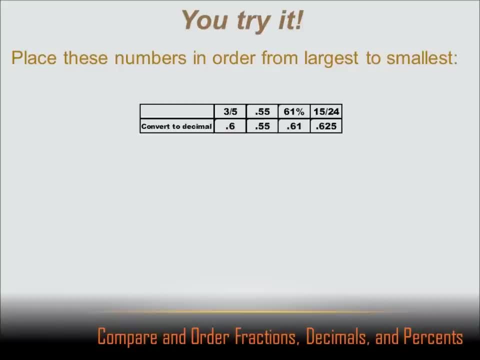 divide 3 by 5 and we get 0.6. we've got nothing to do the 0.55 because it's already a decimal 61%. we move the decimal point 2 to the left and 61% becomes 0.61. and 15 over 24. well, we divide the 15 by 24 and we get .625. 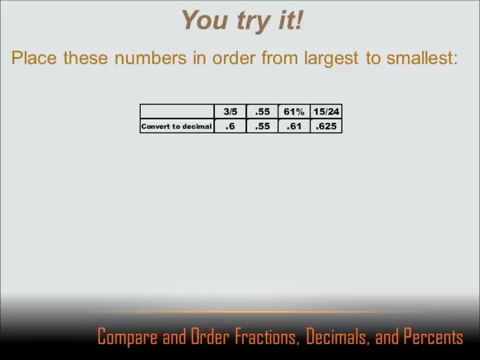 well, now we're comparing apples to apples and not apples to oranges, and it's pretty easy to do. I can see that the largest one is .625, and then .61 is the next largest, and 0.6 and then 0.55.. So the order is 15. twenty-fourths is the largest, 61% is. 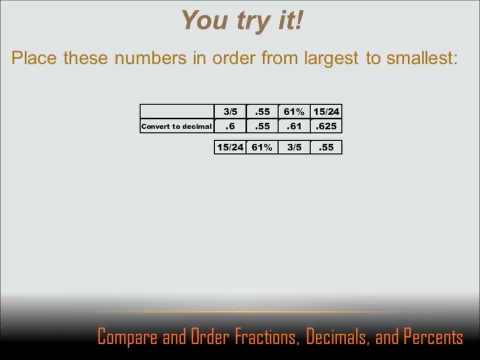 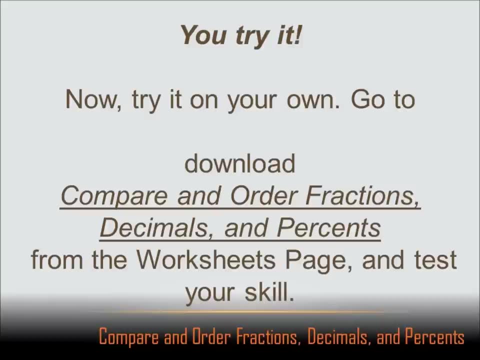 the next, three-fifths is the next and 0.55 is the smallest. Well, we finished our lesson on compare and order fractions, decimals and percentages, and I hope you learned a whole lot. Now it's time to take it a little bit further, Go. 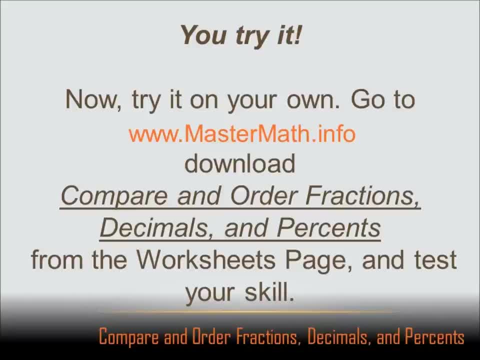 to wwwmastermathinfo and download the worksheet on compare and order fractions, decimals and percents and try your skill there, And then go back to Master Math and try the online quiz and find out if you really know this stuff well. I hope you enjoyed yourself and come back and see us real soon.